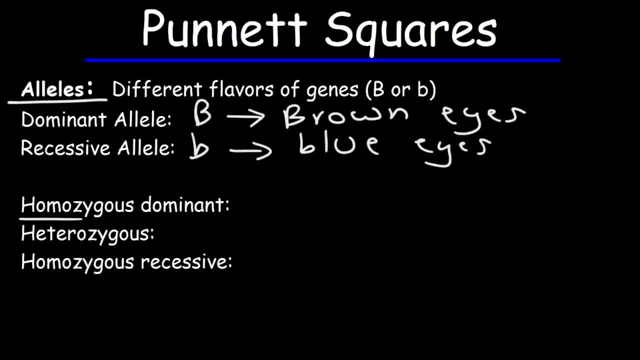 A person with a homozygous dominant trait would have two capital letters or two capital dominant alleles, in this case B and B. Someone who's heterozygous has a dominant and a recessive allele. Hetero means different. 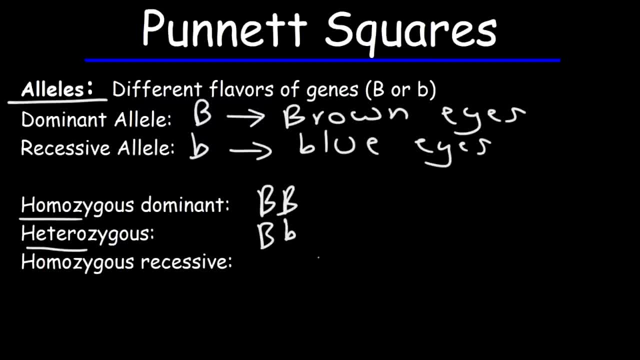 Homozygous recessive. they have the same recessive allele, in this case two lowercase letters. So this information here is referred to as the genotype for that particular trait, because it tells you the genes that correspond to a certain trait. 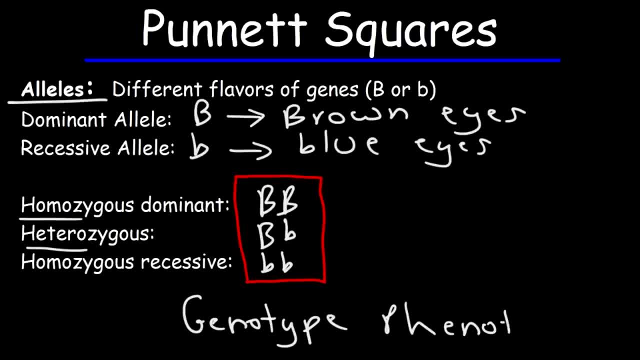 Now the phenotype is associated with the physical characteristics that relate to those traits. Now the individual with the homozygous dominant trait, he's going to have brown eyes, Because big B is associated with brown eyes. The person with the homozygous recessive trait is going to have blue eyes. 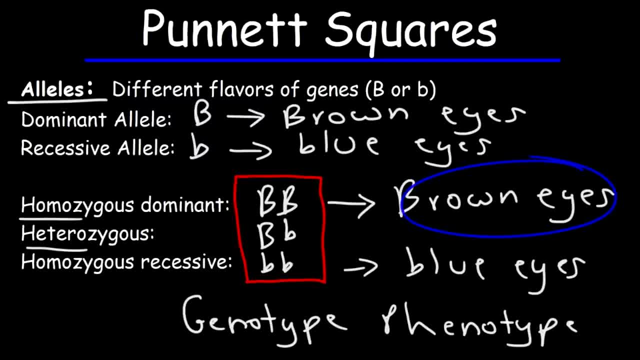 So this represents the phenotype of the individual, the physical characteristics that you can visibly see. Now, what about the heterozygous individual, where he has both the dominant and the recessive allele? What physical characteristic will he display, or she? 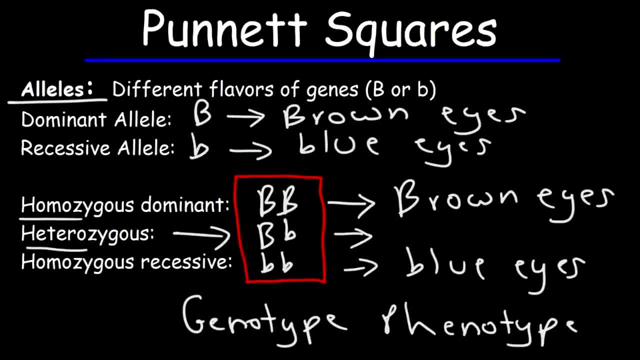 What will be that individual's phenotype. So what would you say? Which one is going to win, the dominant allele or the recessive allele? Whenever you have an individual with a heterozygous trait, the dominant allele is going to win the battle. 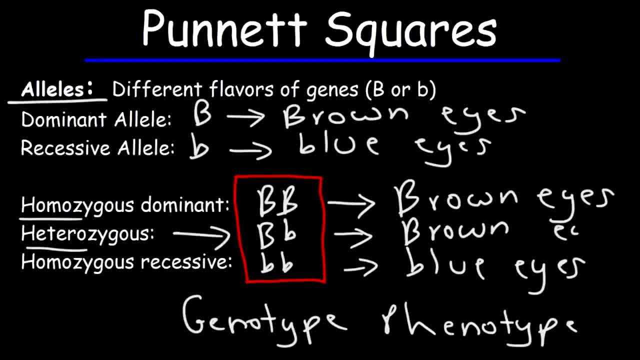 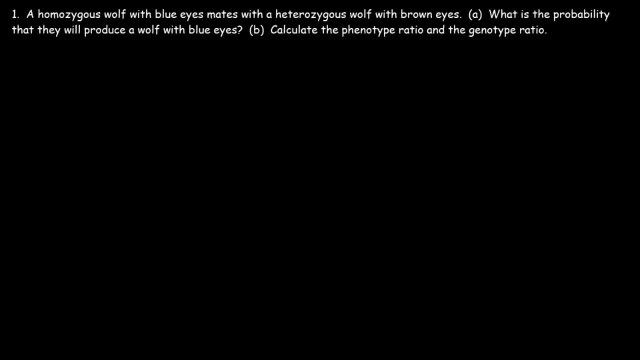 So this person is going to have brown eyes. Let's start with this one: A homozygous woman, A heterozygous wolf with blue eyes, Mates with a heterozygous wolf with brown eyes. What is the probability that they will produce a wolf with blue eyes? 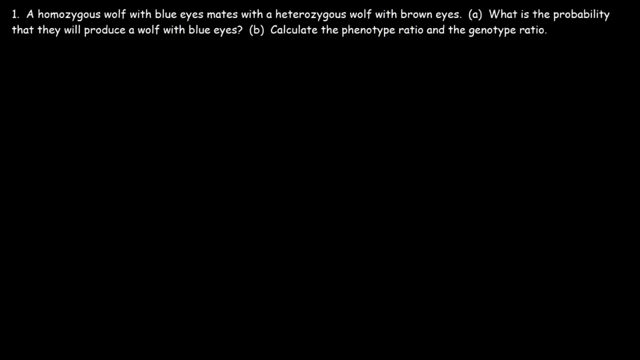 So let's begin by drawing a monohybrid cross. So this is a Punnett square that only focuses on one characteristic, one trait, in this case eye color. So this is a Punnett square that only focuses on one characteristic, one trait, in this case eye color. 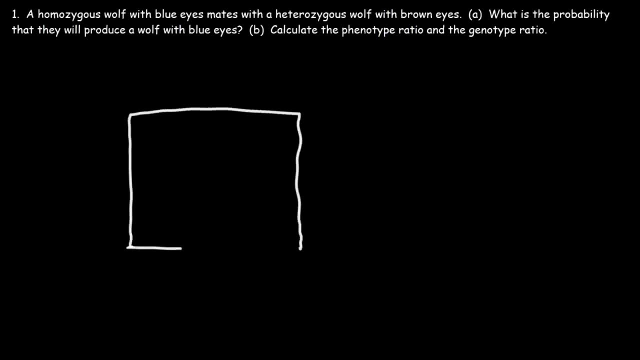 So what we're going to do is we're going to draw one square And then we're going to draw a vertical line and a horizontal line, So now we have a total of four squares. Now, what is the genotype of the homozygous wolf? 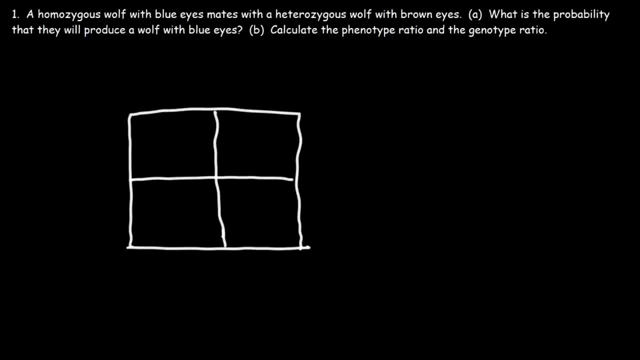 So homozygous means that he has, or it has both the same genes, Either lowercase b Or capital B, But they have to be the same. Now we're dealing with blue eyes and brown eyes. Typically, blue eyes is usually the recessive trait. 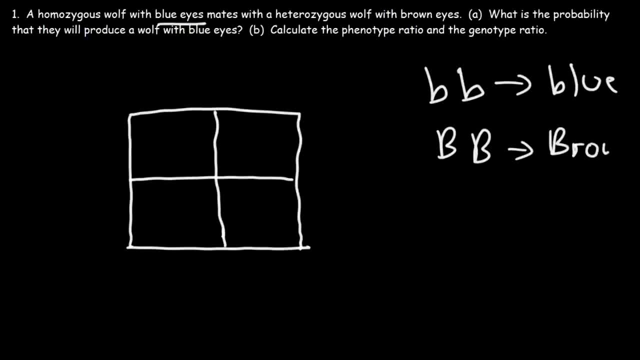 And brown eyes is usually the dominant trait. So here we have a homozygous wolf with blue eyes. So therefore, that wolf has the genotype lowercase b, lowercase b Which I'm going to put here Now. the second wolf is a heterozygous wolf with brown eyes. 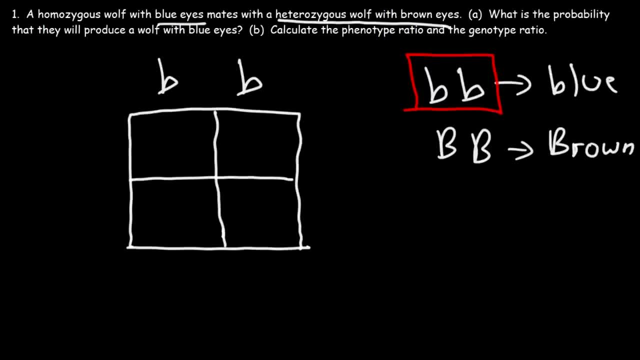 So, based on that information, what is the genotype of that wolf? So it's heterozygous, which means that it's going to have two different alleles, One capital, one lowercase, And it's still going to have brown eyes. 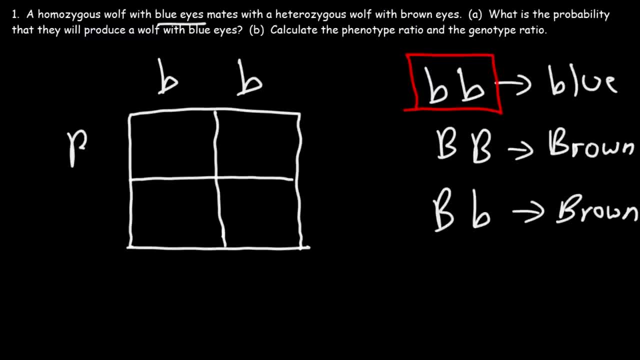 Since capital B is the dominant allele. So now all we need to do is Basically fill in the Punnett square. So in this square we're going to write these two letters And we're going to put the capital letter first. 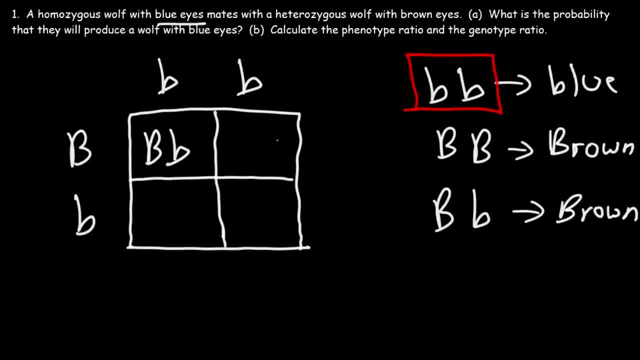 So it's going to be capital B and then lowercase b, And the same is true for this one And for this particular square. it intersects these two letters, So it's going to be lowercase b, lowercase b, And for the last one it will be the same. 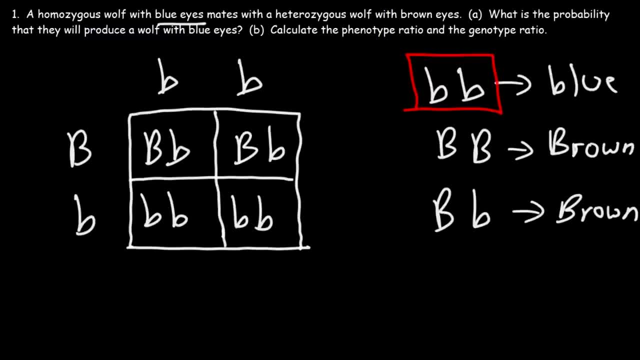 So once we fill out the Punnett square now we can answer. So what is the probability that they will produce a wolf with blue eyes? So this represents the genotype of a wolf with blue eyes And these genotypes represent a wolf with brown eyes. 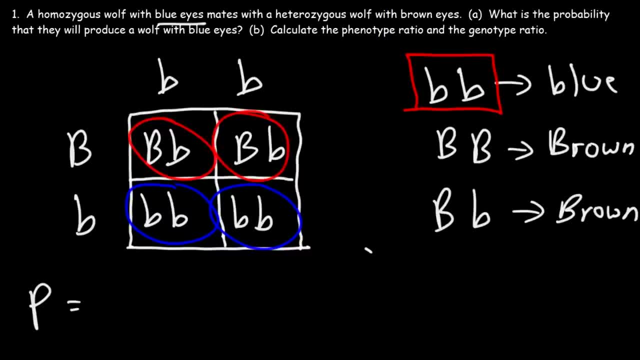 So to calculate the probability, you look at how many have been chosen. In this case there's two with blue eyes Out of a total of four. So two out of four, that's one half, which is 50%. 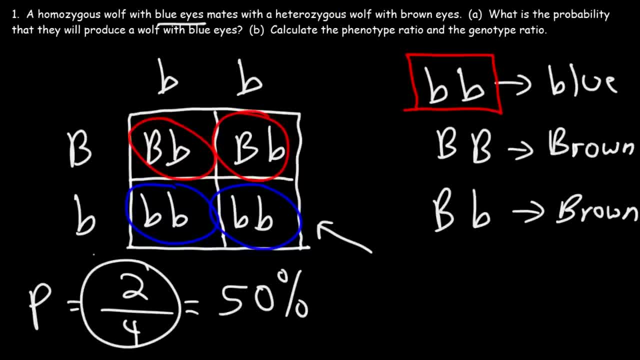 If you divide this, you'll get 0.5 in your calculator And then multiply that by 100.. That will give you 50%. So that is the probability that they will produce a wolf with blue eyes. Now what about part B? 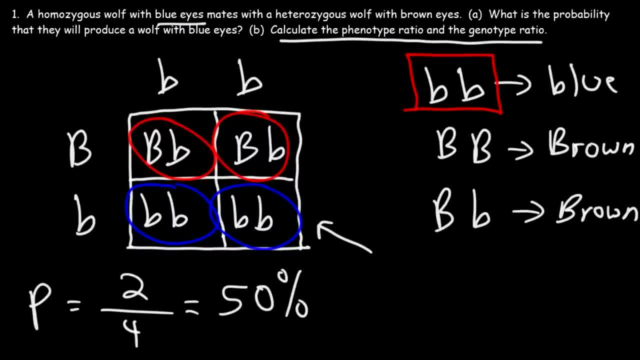 Calculate the phenotype ratio and the genotype ratio. So let's make some space. So let's start with the phenotype ratio. So we're dealing with the colors of the eyes, the physical characteristics, And there's only two colors to deal with. 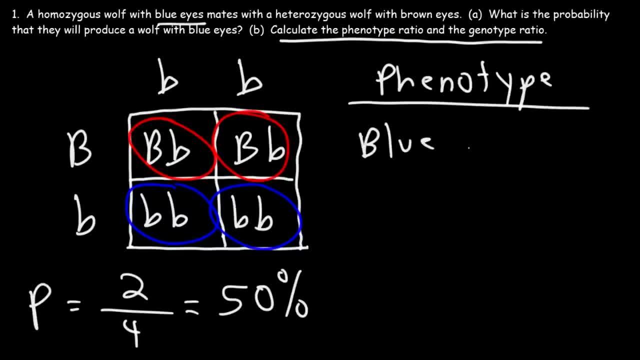 Either the baby wolves have blue eyes or they have brown eyes. So out of, let's say, four baby wolves, two of them will have blue eyes And two will have They'll have brown eyes, which I use the color red instead of brown, for some reason. 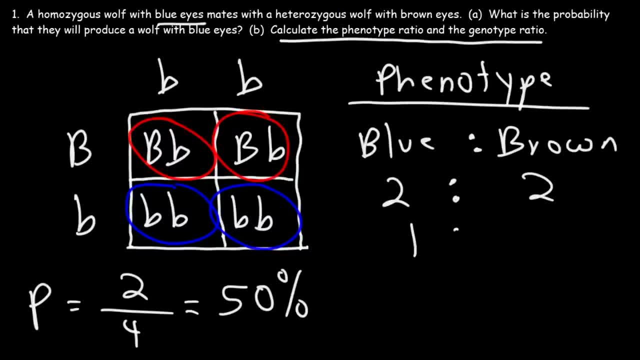 And so you can divide both numbers by two, And thus you get the simplified ratio. So it's a one-to-one ratio. So that's the phenotype ratio: Blue to brown, or, if you want to do, brown to blue. it's still going to be one-to-one. 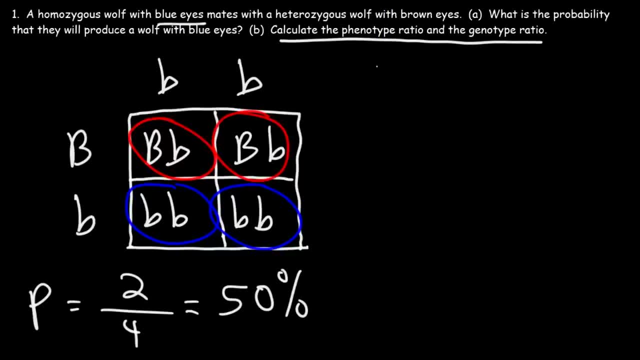 Now let's talk about the genotype ratio, And it's only two genotypes, So it's either big B and little b, which we see here, or little b and little b, So it's still two to two which can be reduced to a ratio of one-to-one. 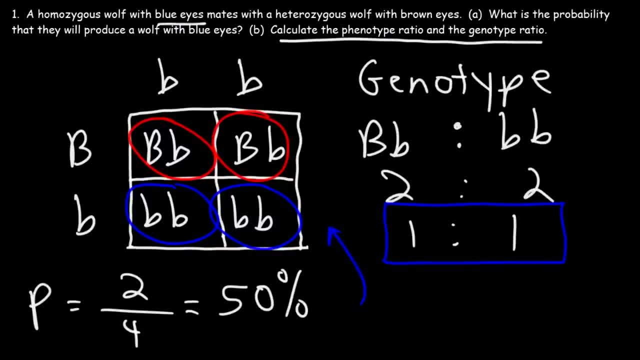 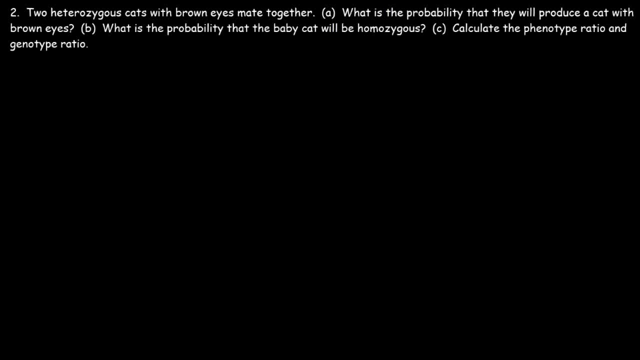 So that's the genotype ratio for the first generation. Now let's work on another example: Two heterozygous cats With brown eyes made together. What is the probability that they will produce a cat with brown eyes? So once again we're going to say capital B is associated with brown eyes. 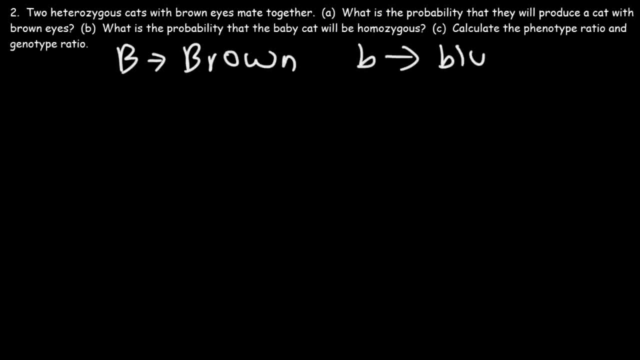 And little b is going to be associated with blue eyes. So, based on this information, calculate the probability that the baby cat is going to have brown eyes. So let's begin, And by drawing a Punnett square. Now, the fact that both parents are heterozygous means that their genotype is big B, little b. 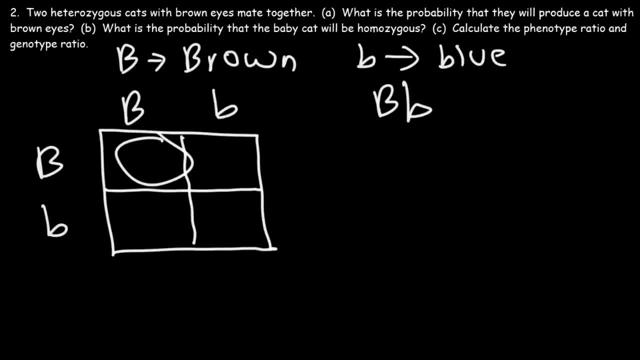 So we can write that here. So in this spot that's going to be the intersection of big B and big B. Here we're going to have big B, little b, Same over here, And for the last one that's going to be the intersection of two lower. 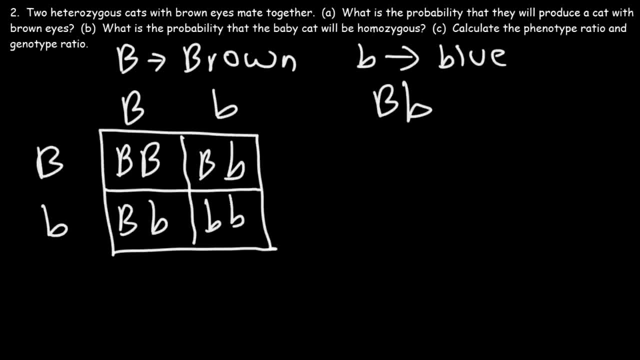 K is B's, So now we can focus on answering the question. What is the probability that they will produce a cat with brown eyes? So which cats will have brown eyes? So this one will be brown, And the same is true for these two. 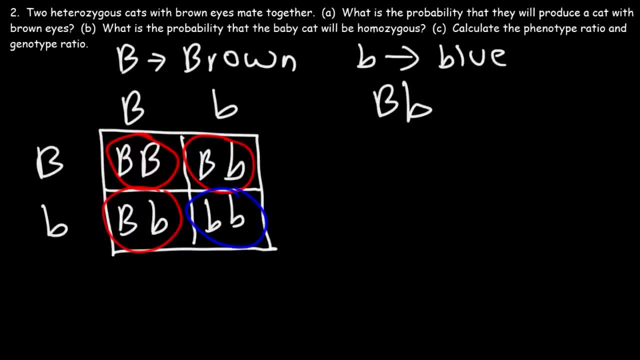 And this particular cat will be blue. So out of four, we're going to have two. So out of four, we're going to have two. So out of four cats, three of them will have brown eyes. So the probability will be the three cats with brown eyes out of a total of four. 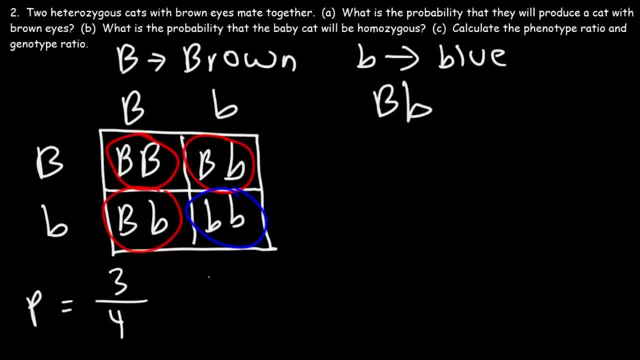 Three divided by four is 0.75.. If you multiply that by 100, you're going to get 75%. So that is the probability that they will produce a cat with brown eyes. Now part B: What is the probability that the baby cat will be homozygous? 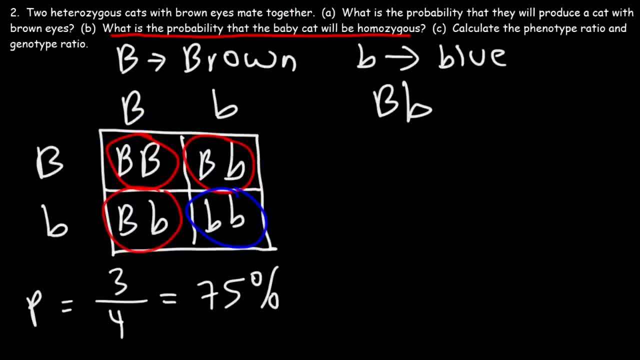 So out of all the traits listed here, which one is homozygous? So homozygous means that they have the same letters. In this case it's big B and big B. That's homozygous, or little b with little b. 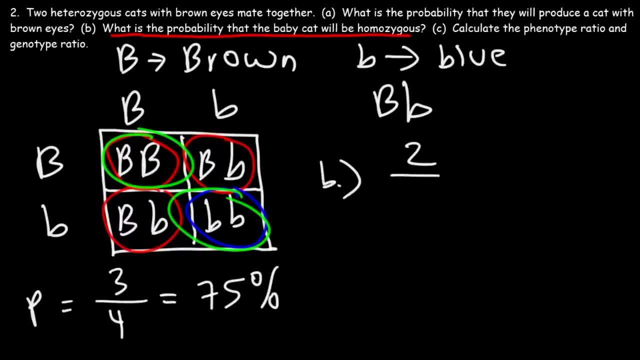 So for part B there's going to be two cats out of a total of four with a homozygous trait or a homozygous genotype. So that's 50%. Now let's talk about calculating the phenotype and the genotype ratio in part C. 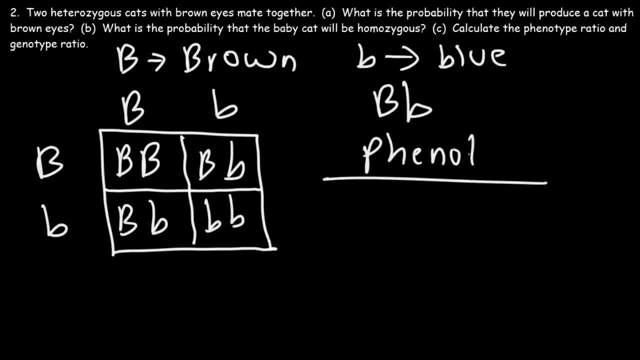 So let's start with the phenotype ratio. So once again we only have two colors, two eye colors, So that's brown and blue, And we have three genotypes that correspond to the color brown And only one that corresponds to the color blue. 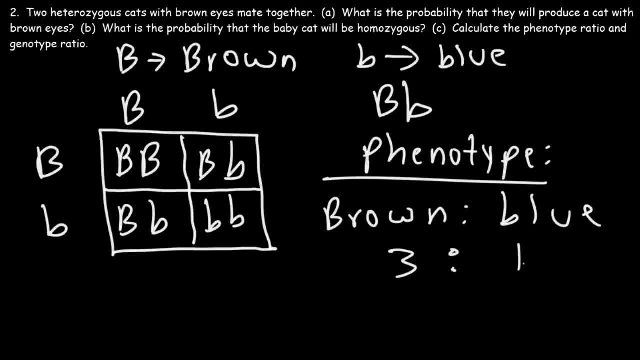 So it's going to be three to one. So that's the phenotypic ratio. Now let's calculate the genotypic ratio. So first let's list the different types, the different genotypes that we see. 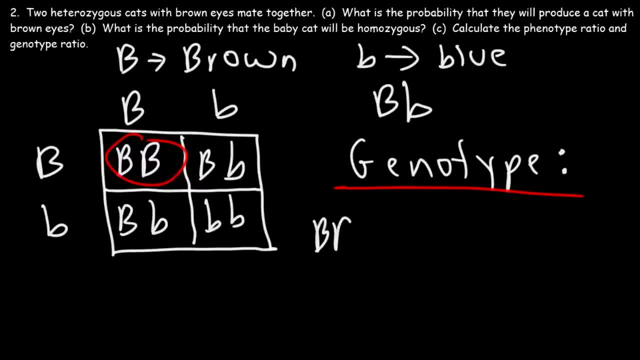 So this is one Big B and big B. These two are the same- Capital B and lowercase b- And this one is the last one remaining. So we only have one homozygous dominant genotype And we have two heterozygous genotypes. 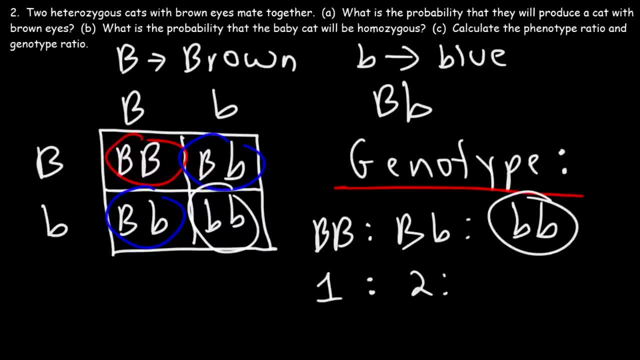 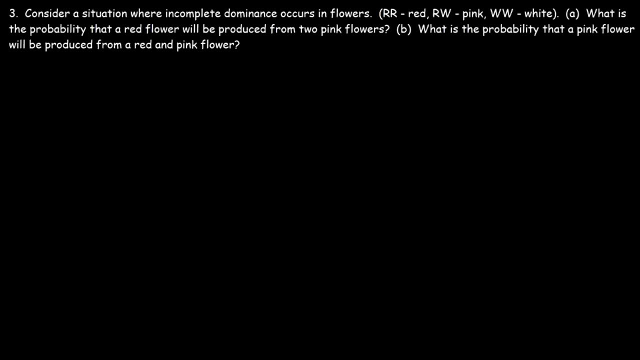 And one homozygous recessive genotype. So the genotypic ratio is one to one. Number three: Consider a situation where incomplete dominance occurs in flowers. So capital R is associated with red, Capital W is associated with white. 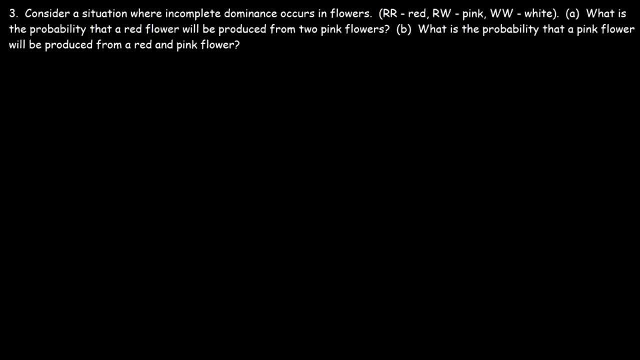 But when you have a heterozygous genotype RW, you get something in between, In this case the color pink. So with that in mind, let's answer the question for part A. What is the probability that a red flower will be produced from two pink flowers? 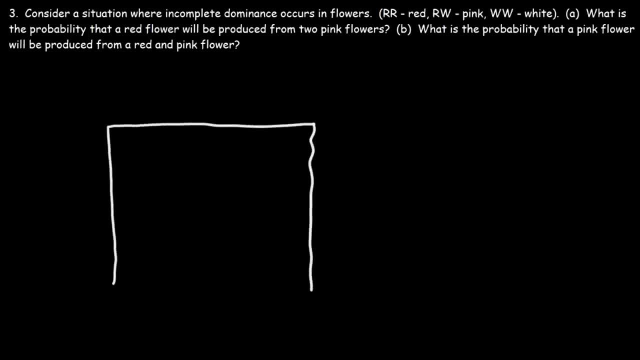 So we're only dealing with one trait. So we just need a Punnett square, A two by two Punnett square, with four squares inside, So each pink flower will have the genotype RW. Now let's go ahead and fill the table. 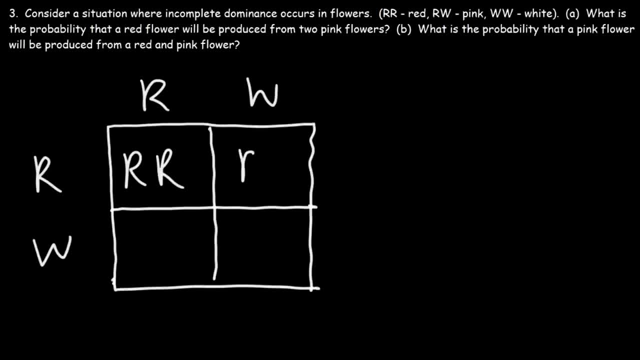 So this is going to be RR, RW, RW and WW. So what is the probability that a red flower will be produced? So this is going to be a red flower. Here we're going to get a white flower. 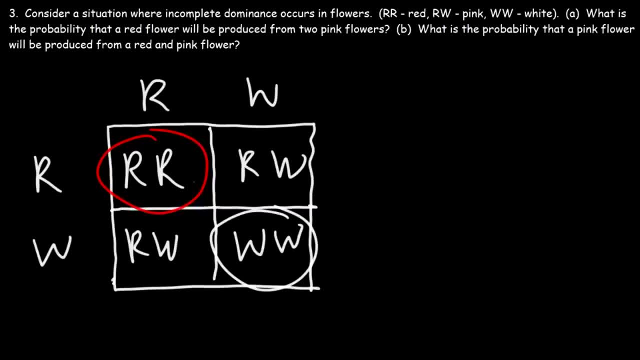 And let me look for a pinkish color, So these two will be. they're going to be pinkish, So these two will be. they will represent the pink flower, So we have a total of two. well, we're looking for red flowers. 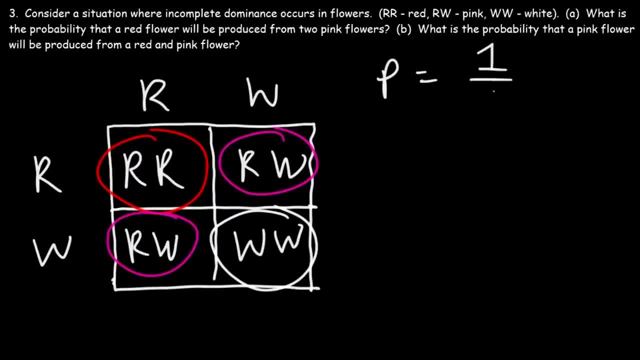 So we only have a total of one red flower out of four. So one divided by four is 0.25 times 100.. So that gives us a probability of 25%. So there's a 25% chance that a red flower 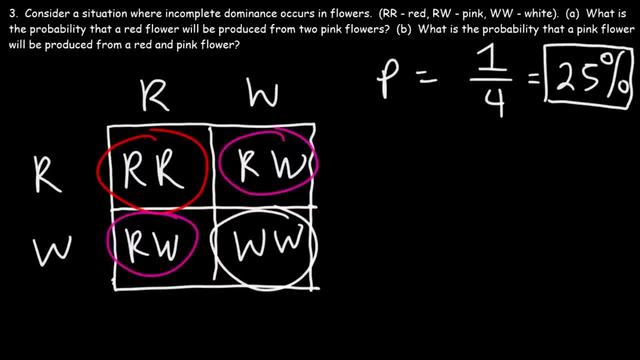 will be produced from the two pink flowers. If we wish to calculate the probability that a pink flower will be produced, it's going to be 2 out of 4. And so that's going to be 50%, And the probability of getting a white flower is just 1 out of 4, which is 25%. 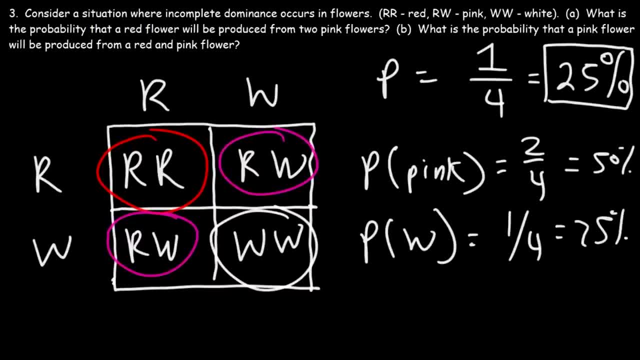 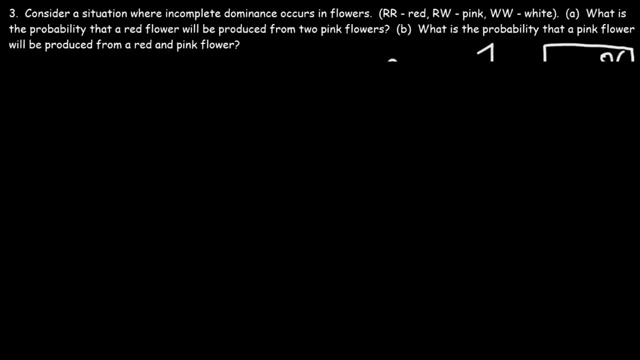 Now let's move on to Part B. What is the probability that a pink flower will be produced from a red flower, Red and pink flower? So we no longer have two pink flowers For the parents. we have one red, one pink. 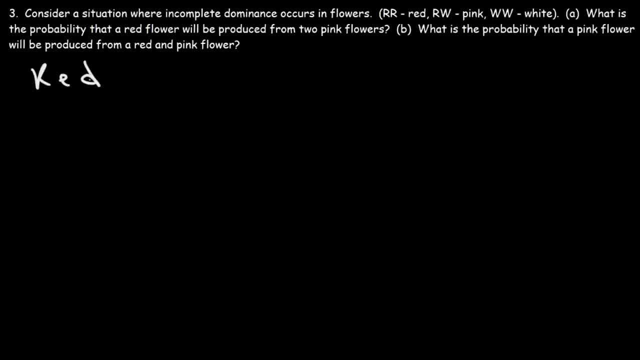 So let's write the genotype. So the genotype for the red flower will be RR, And for the pink flower it's going to be RW. So RW for pink, RR for red. So let's go ahead and fill out the square. 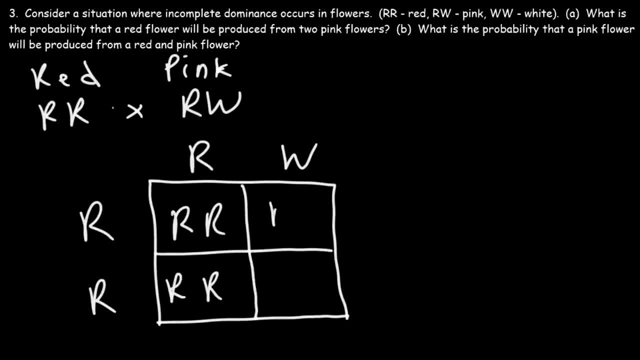 So this is going to be RR And then we're going to have RW, So these two flowers will have a red color And these two will have a pink color. So the probability that a pink flower will be produced. 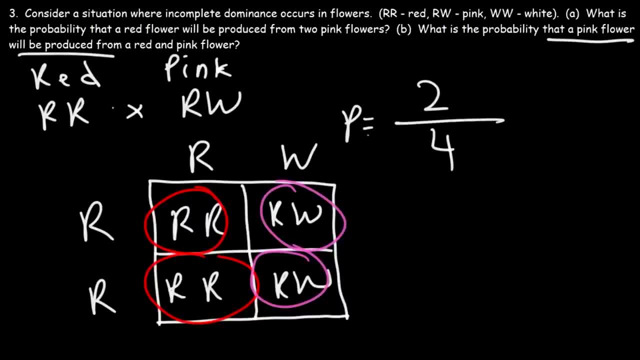 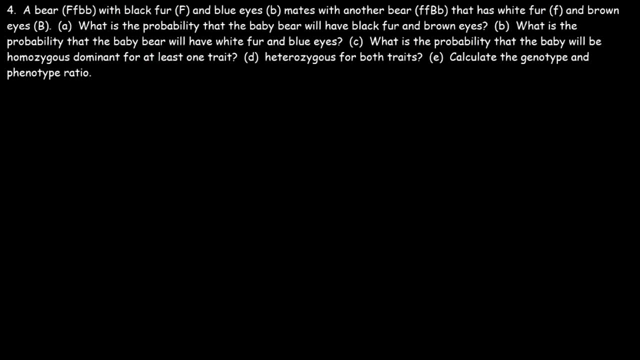 there's two pink flowers out of a total of four, And so that's going to give us a 50% probability. So that's it for Part B, Number 4.. A bear with black fur and blue eyes mates with another bear that has white fur and brown eyes. 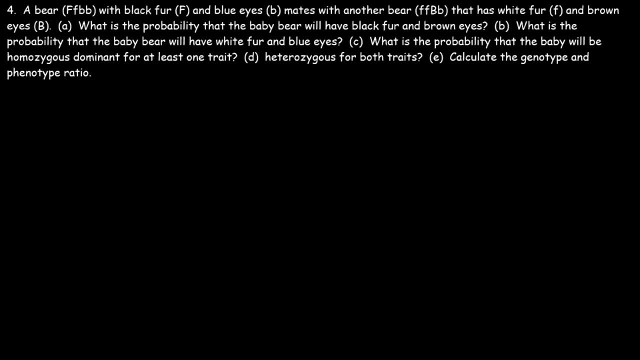 What is the probability that the baby bear will have black fur and brown eyes? So in the last three example problems we only dealt with one particular characteristic, So we used a monohybrid cross. But in this problem we're dealing with two traits. 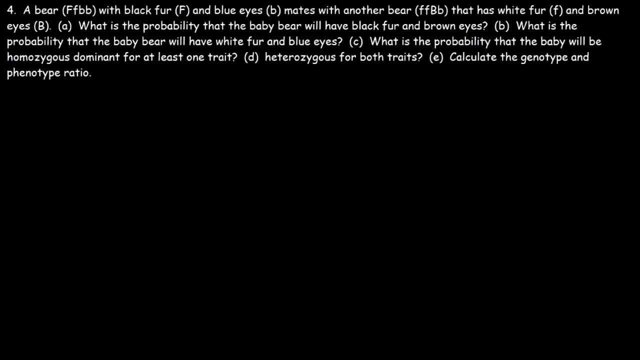 The color of the fur and the color of the eyes. So we need to use a dihybrid cross. So this problem will involve more work. So let's begin by drawing a Punnett square. Hopefully this is big enough. 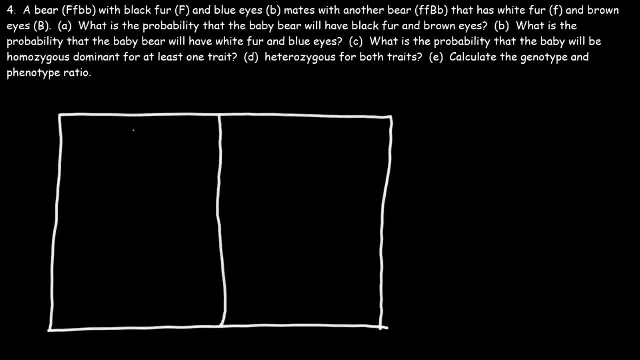 And this one is going to have four columns and four rows. So 4 times 4 is 16.. And so we're going to have a total of 16 squares. Now the genotype for the first parent is going to be: 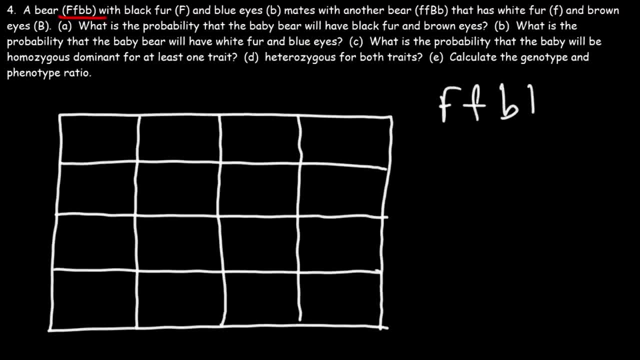 big F, little f, little b, little b. And the genotype for the second parent is going to be little f, little f, big B, little b. Now what should we place here and here? Here's what you shouldn't do. 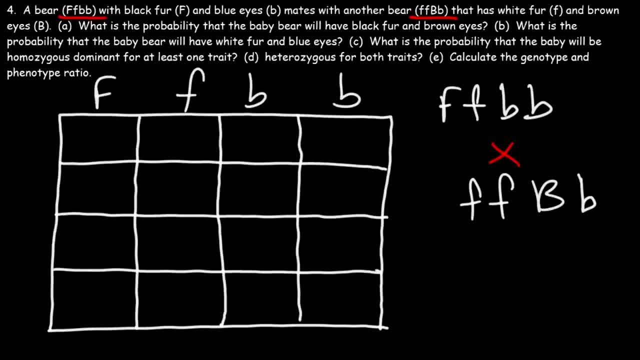 You shouldn't just write one letter In each column. This is not the right way to do it, Because you're dealing with two characteristics, So you need to place two letters in each column, So that in each box you're going to get four letters. 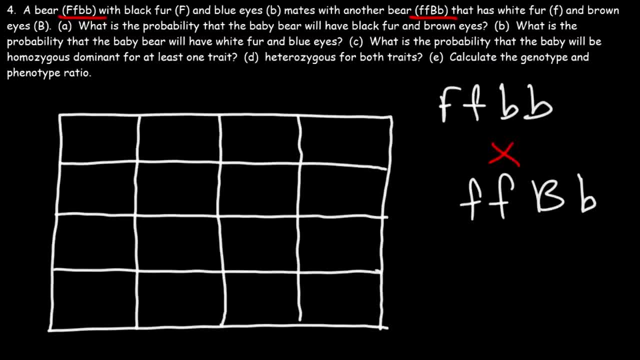 So how do we know which two letters go where? So, hopefully you've taken algebra and you remember how to FOIL And that's what we're going to do. So we're going to take one letter from the first box. 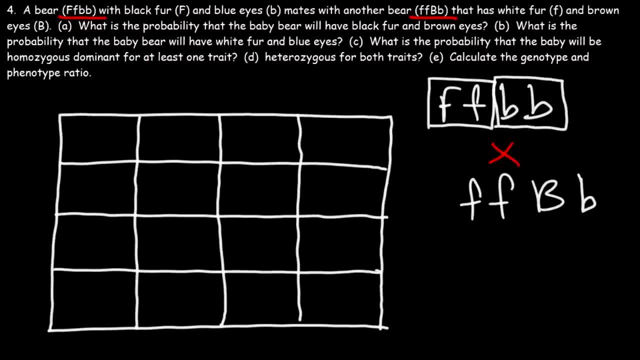 and pair it up with a second letter from the second box that represents the second characteristic. So we're going to pair up capital F with lowercase b, So that's going to give us big F, little b. And then we're going to pair up 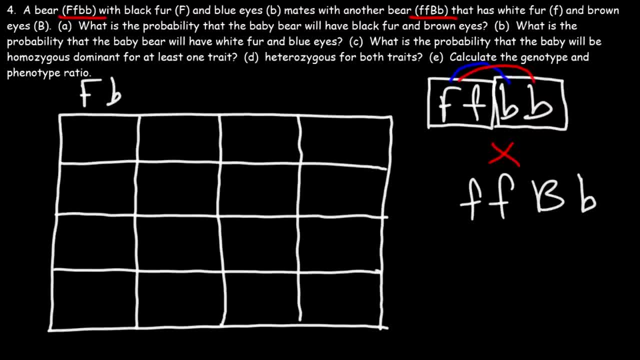 big F and little b again. So if you remember the word FOIL, it's first, That's for the blue line And for the red line outer. So that's going to be big F, little f, And then i for inner. 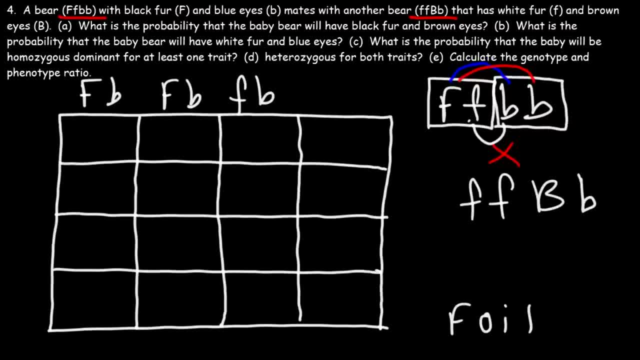 Little f, little b, And then the last Little f, little b again. Now let's do the same thing for the second genotype, Or the genotype for the second parent. So it's going to be little f and big B. 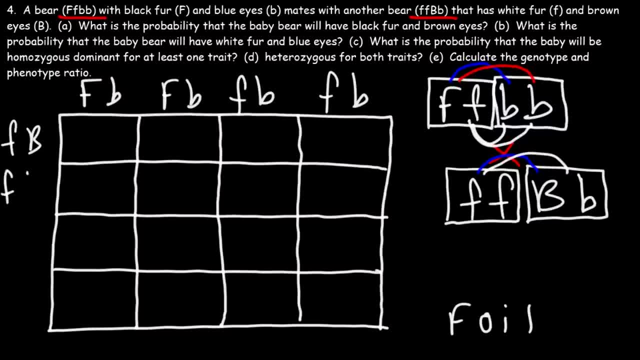 And then we have little f, little b, And then it's going to be little f, big B And little f, little b. So now let's fill in the Punnett Square. So we have big F, little f. 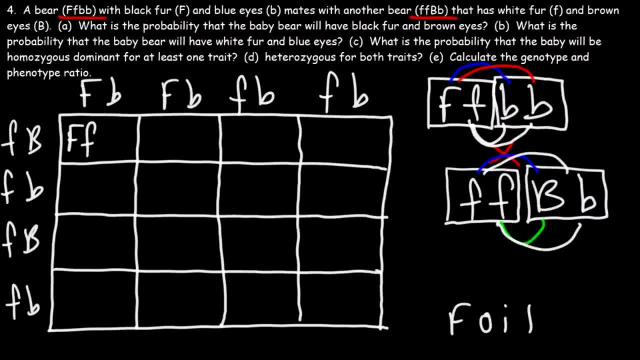 And then big B, little b. So this is going to take a while. What I recommend doing is pausing the video and fill it out yourself, And then you can play the video again and see if you have what I have as well. 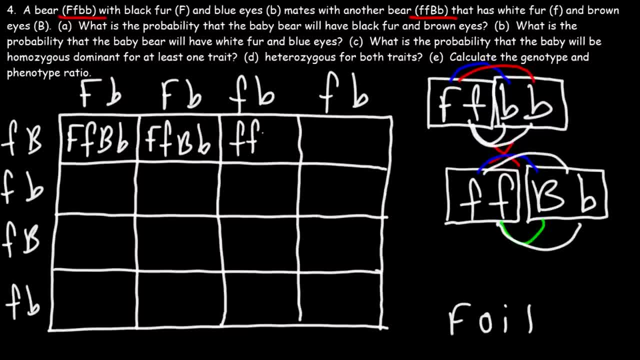 So I'm just going to take a minute and fill everything out. So I'm going to try to double check my work as I do this So I don't make any mistakes. Almost done. You can fast forward this if you want to. 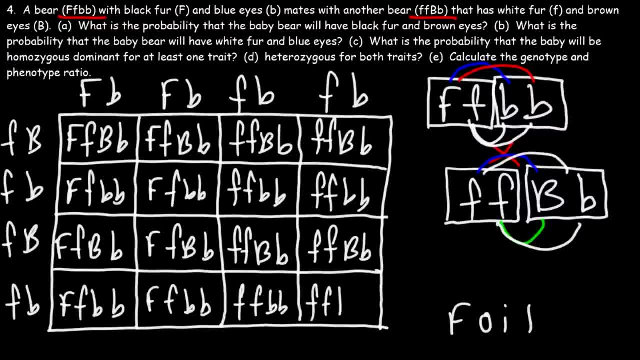 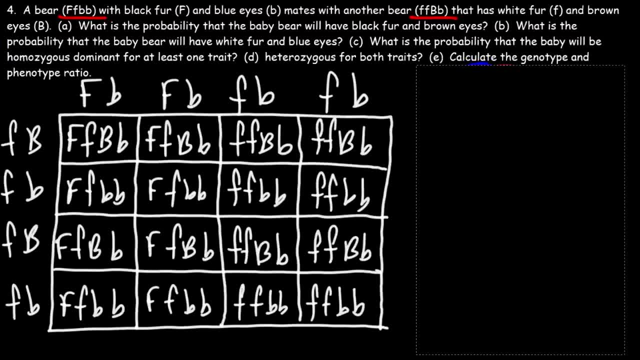 So now, at this point, we can answer part A. So what is the probability that the baby bear will have black fur and brown eyes? So I'm going to use- I can't use- black because the background is black- 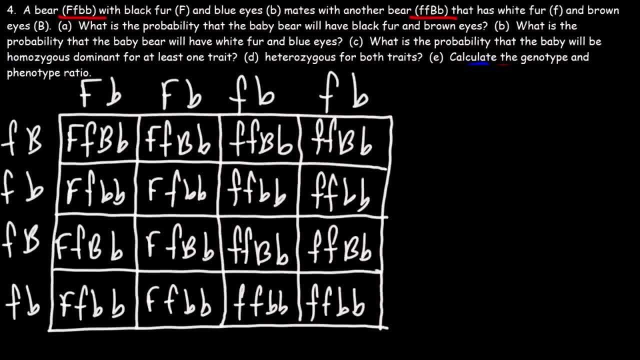 So I'm just going to use like blue for black. So black fur is capital F. All we need is just one capital F. So let's identify every genotype that will show up with the black fur physical characteristic. So all we need is just one capital F. 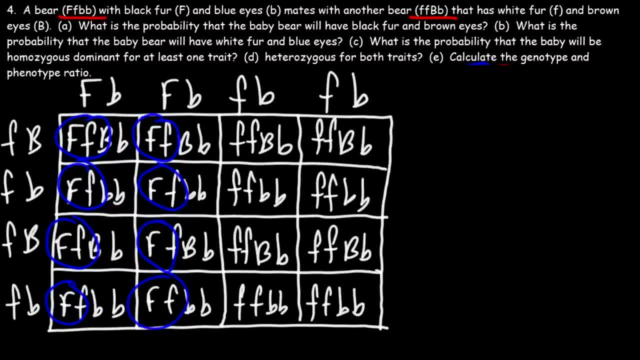 And the bear will have black fur. Now let's identify all the bears that will have brown eyes. So all we need to identify is at least one capital B And that's it. So now we need to identify all the bears. 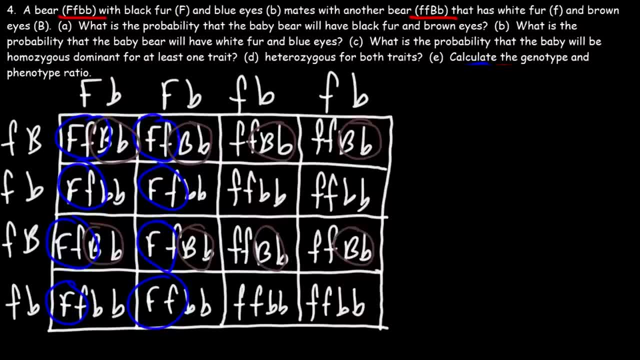 that have both black fur and brown eyes. So this is one, Two, Three And four, So we have a total of four. Well, there's four that's been selected out of a total of sixteen possibilities, because there's a total of sixteen squares. 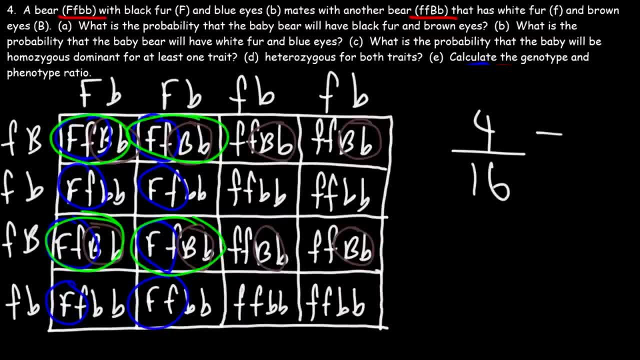 So four out of sixteen. If you divide both numbers by four, you can reduce the fraction to one over four, which is .25 or 25%. So this is the probability that the baby bear will have black fur and brown eyes. 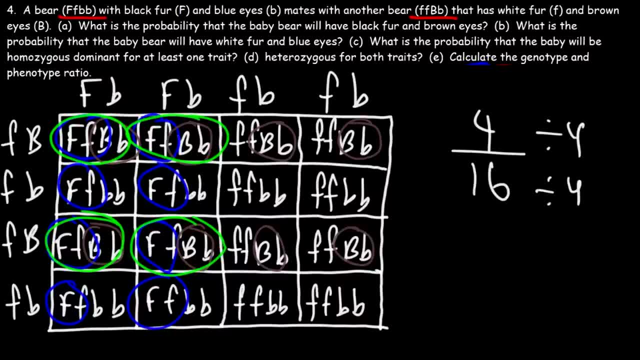 So now let's move on to part B. What is the probability that the baby bear will have white fur and blue eyes? Go ahead and try that. So let's identify all the bears with white fur. So that means that they need to have. 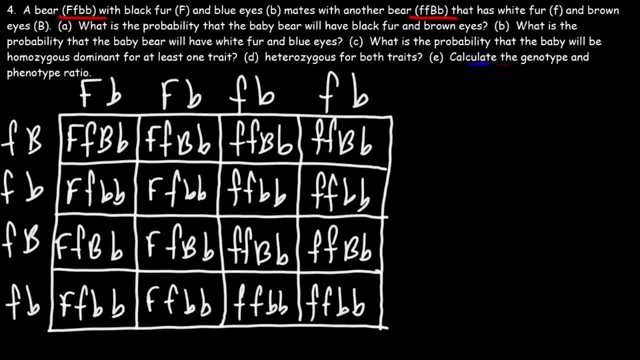 the genotype lowercase f and lowercase f. So this bear has white fur. This one too. Basically all the ones on the second half of the Punnett square, they will all have white fur because they're homozygous, recessive. 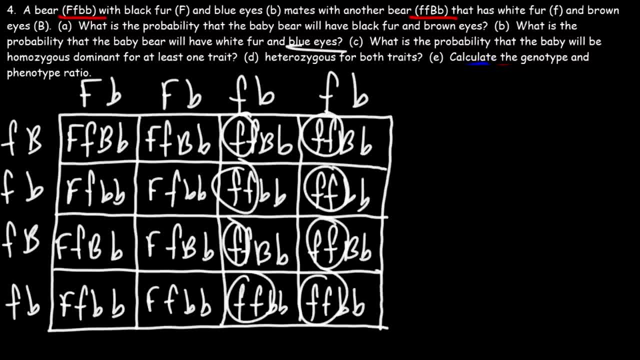 Now let's identify all the bears with blue eyes. So they should have the genotype little b. little b, since blue eyes is going to be the recessive trait or the recessive allele. So let's use the color blue. So here's one. 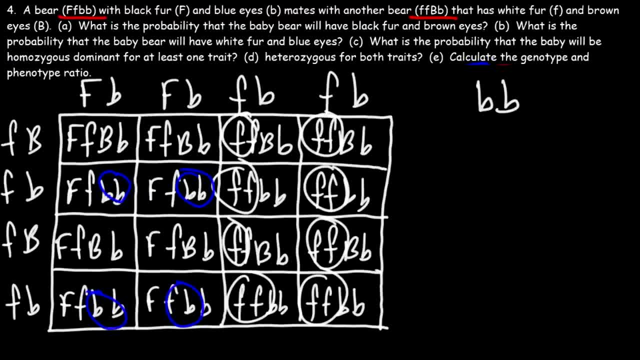 Here's another one, That's another one And that's it. So the bears that have both white fur and blue eyes is one, two, three, four. So once again, it's four out of sixteen, which is one-fourth. 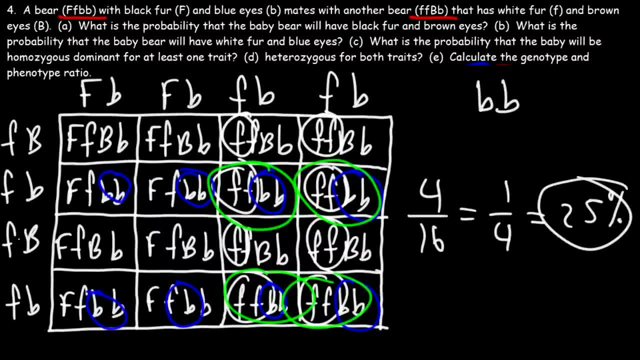 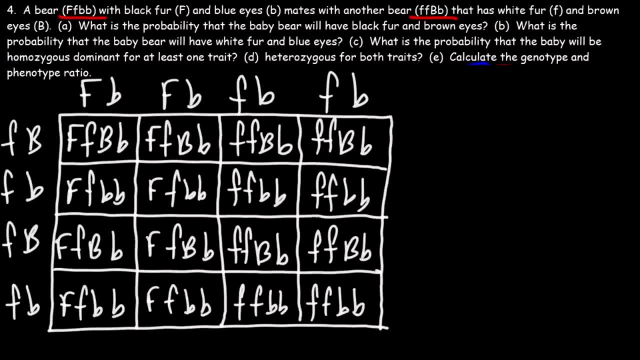 And so the probability is 25%. Now let's move on to part C. So what is the probability that the baby will be homozygous, dominant for at least one trait? So let's think about what that means. 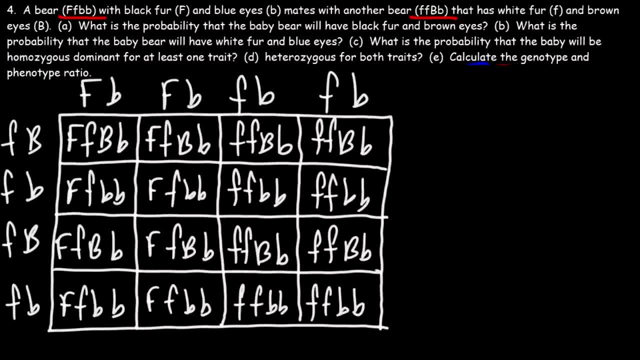 Homozygous dominant. So that means that they have to have the same alleles, either big F, big F, little f, little f, big B, big B, little b, little b. Now, so those are the homozygous genotypes. 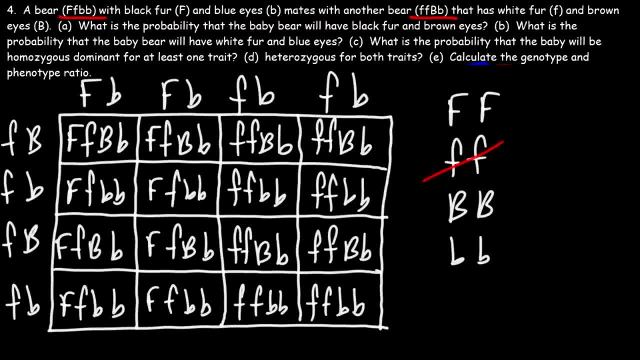 Now we want the dominant ones, not the recessive ones, so we can eliminate these two. So we either want big F and big F, or big B and big B. So let's see if we can identify any of those. 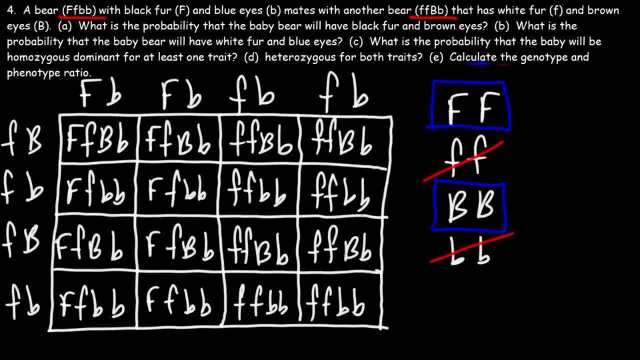 And I don't see it at all. So the probability is 0% because there's none with a homozygous dominant trait. Now part D: What is the probability that it's going to be heterozygous for both traits? 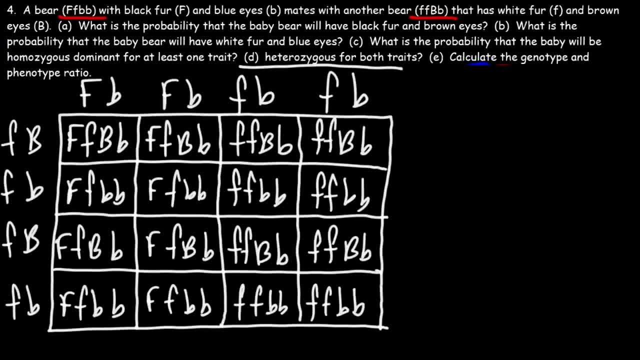 So heterozygous means that we're going to have one big letter, one little letter. So for the first trait it's going to be big F, little f. For the second trait, big B, little b. So here is one. 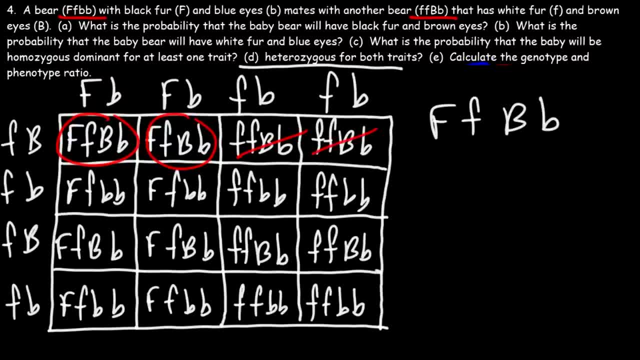 Here is the second one. That doesn't count, Not those. Here's another one, And not those as well. So once again, it's 4 out of a total of 16, which seems to be 25%. 25% is the number of the day. 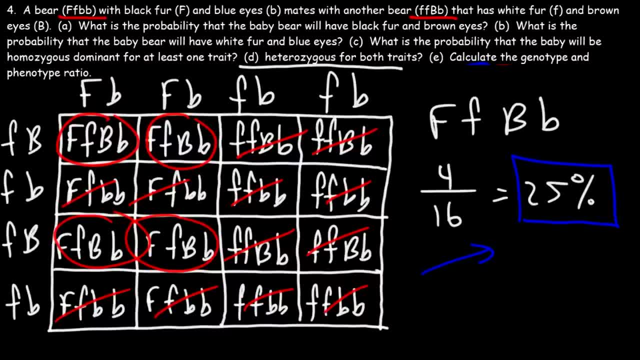 We're getting this answer a lot. So that's the probability that the baby bear will be heterozygous for both traits. Now let's move on to part E. So we need to calculate the genotype and the phenotype ratio. 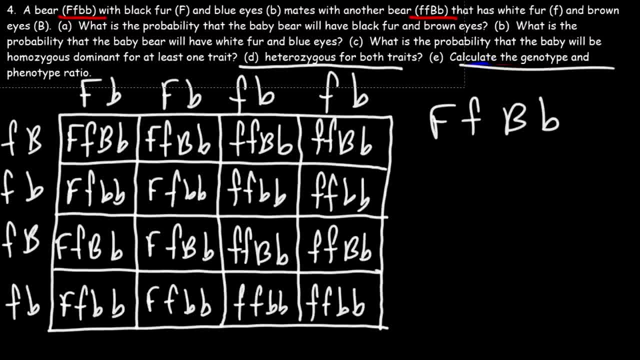 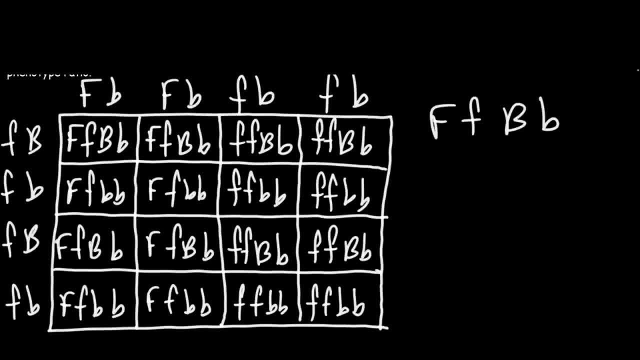 So what I need to do is make some space. So let's start with the genotype ratio. So this is the first one: Big F, little f, Big B- little b, And so let's identify each one with those characteristics. 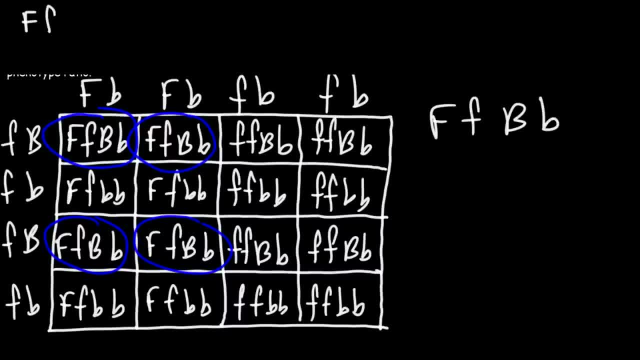 So it's just 4.. Now the next one is little f, little f, Big B, little b, And I see 4 of those, And then the next one is going to be big F, little f, Little b, little b. 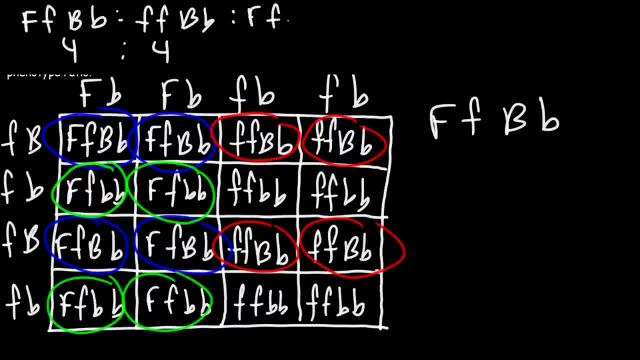 And so there's also 4 of those, And finally little f, little f With little b, little b. So 4, 4,, 4, 4.. If we divide everything by 4, then the genotypic ratio. 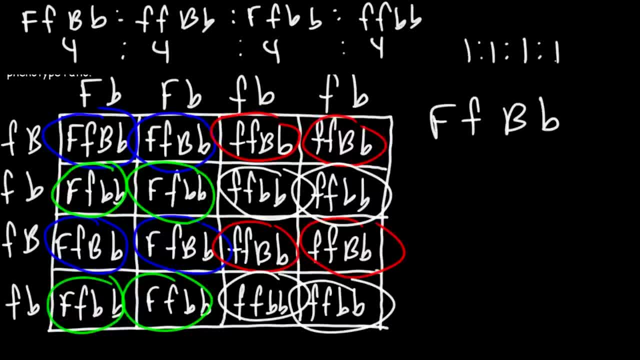 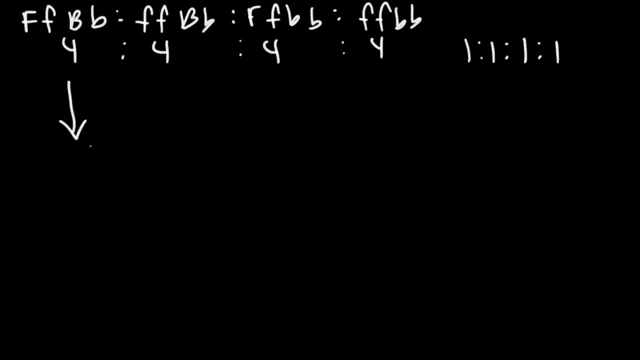 is 1 to 1 to 1 to 1.. Now the phenotypic ratio, the characteristics. it turns out. it's going to be the same. Now the genotype: big F, little f. big B, little b. 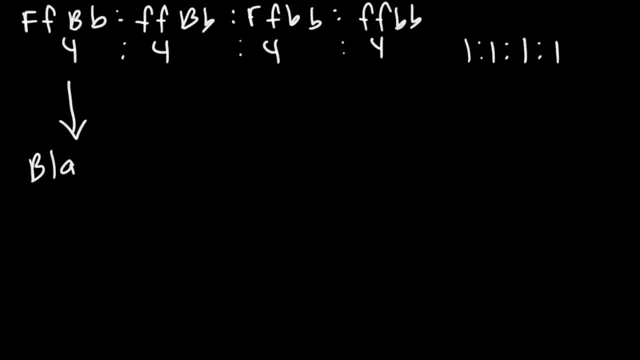 it corresponds to a bear with black fur and blue eyes. Actually, not blue eyes, but brown eyes Because of big B. Now the second genotype, little f. little f, that's for white fur. big B, little b.